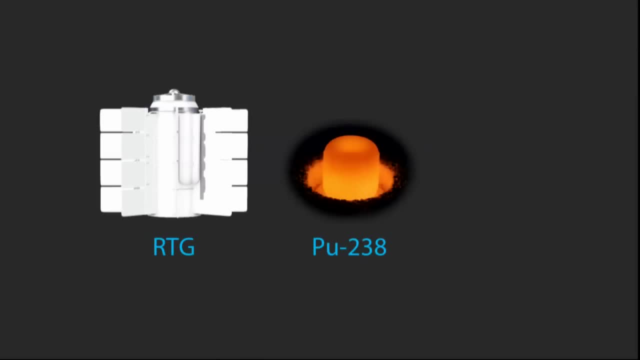 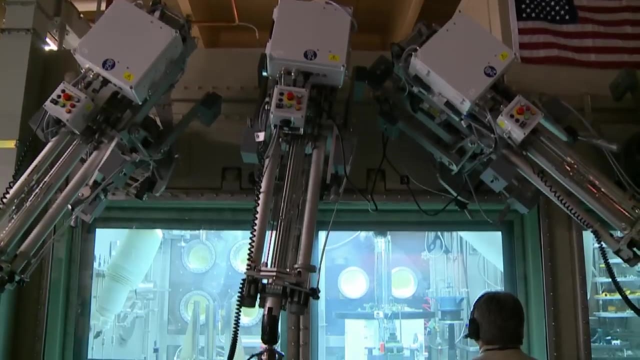 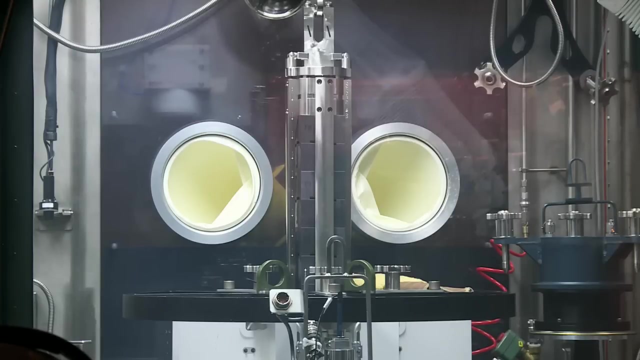 RTGs are devices that turn the heat from the radioactive decay of plutonium-238 directly into electricity. For roughly 15 years, experts at Idaho National Laboratory have played an integral part in fueling and testing RTGs for NASA. Now INL is helping NASA prepare for another mission: the Mars 2020 rover. 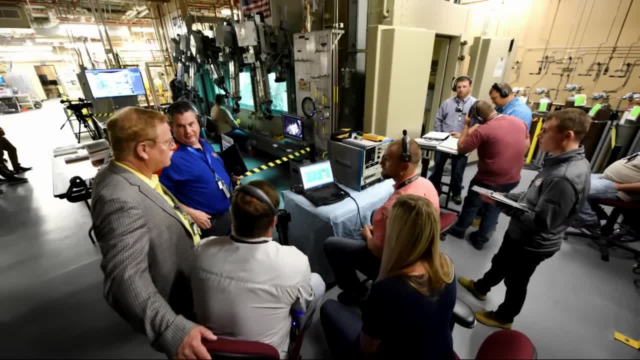 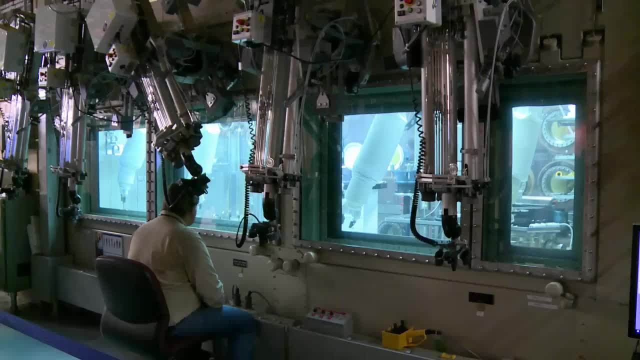 Here's a snapshot of how we fuel and test the rover's RTG. First, the unfueled RTG is removed from its shipping container and tested for integrity. It then moves into a glove box where the radioactive fuel can be safely inserted. 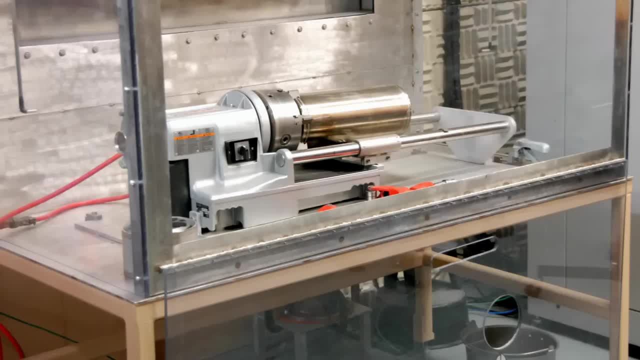 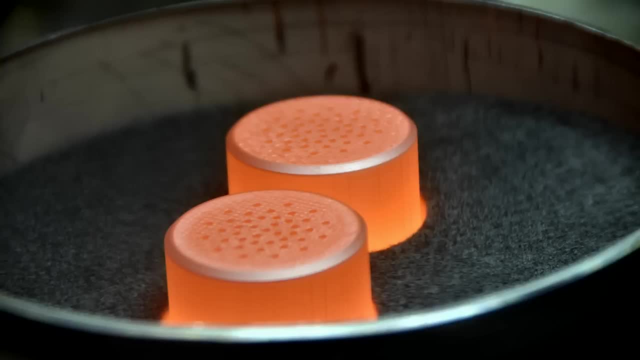 The fuel is shipped from Los Alamos National Laboratory to INL in several layers of shielding In a protective glove box. experts place fueled clads into a graphite housing called a general-purpose heat source. Four fueled clads go into each heat source. 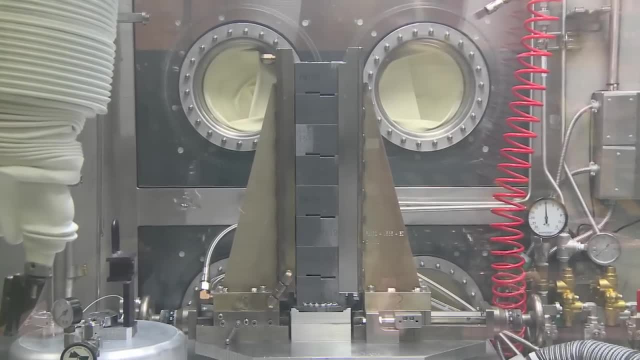 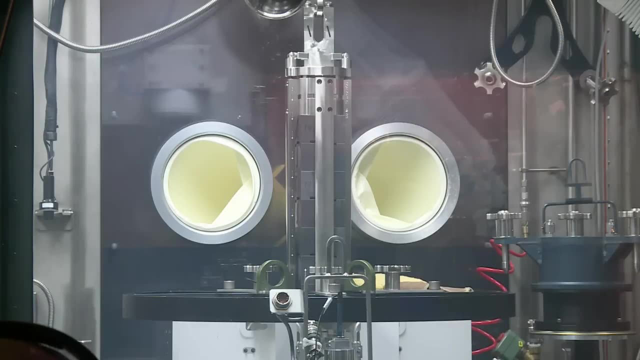 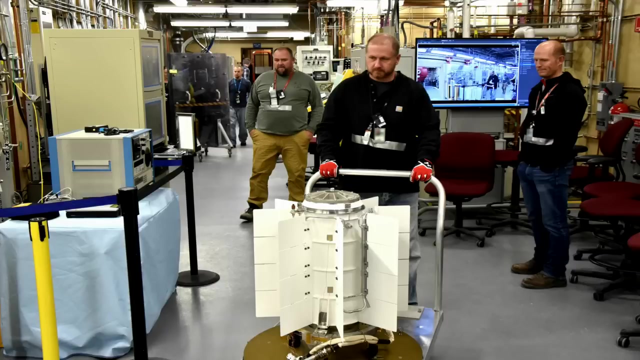 The RTG, designed for the Mars 2020, requires eight general-purpose heat sources, which are stacked on top of each other. Once the RTG is fueled, experts remove it from the glove box to prep for tests that will simulate environments the rover will experience during its mission. 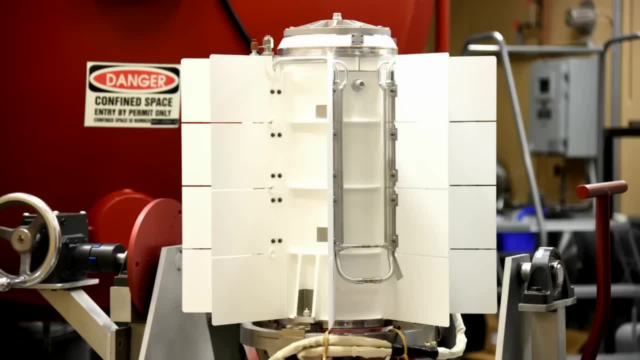 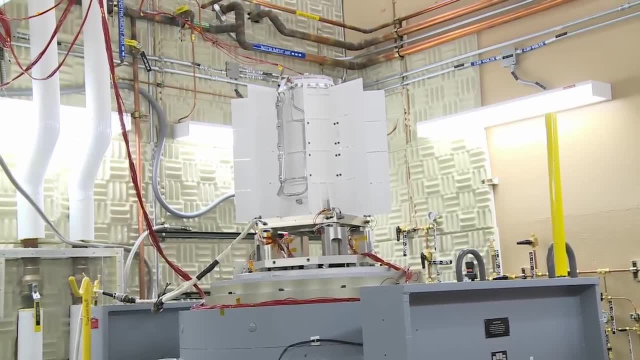 First, electrical and radiation measurements confirm the RTG's power output and radiation field. Then it's transferred to a special room for vibration testing. A large machine vibrates the RTG in three dimensions. To do this it needs to be tested. 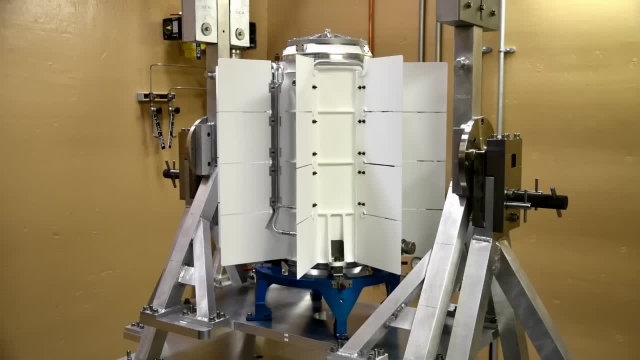 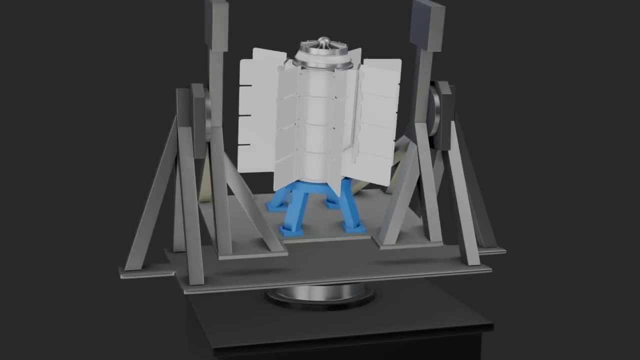 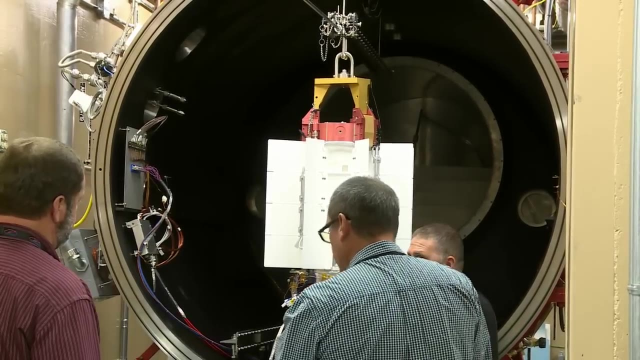 To mimic the shaking that it will experience during liftoff. Next, a series of tests determine the RTG's mass and center of gravity, so that NASA experts will know how it will ride in the rocket and on the rover. The final test determines how well the RTG performs in the vacuum of space. 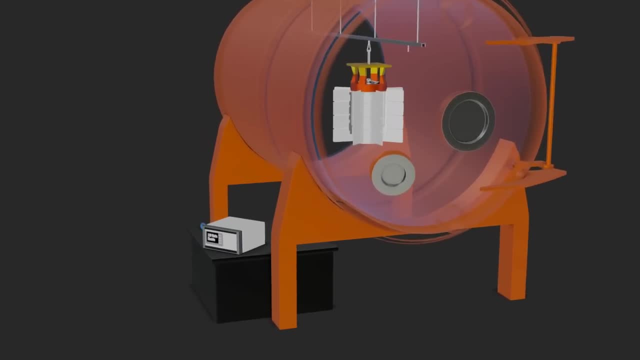 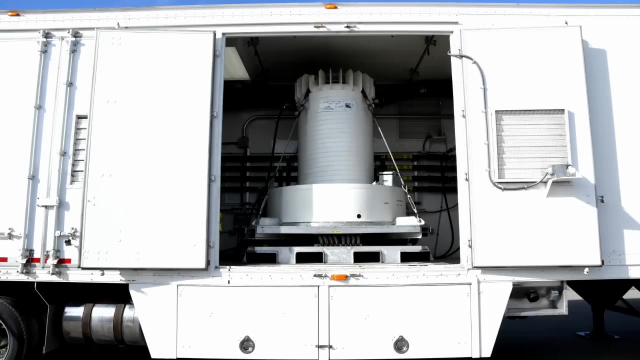 Inside the thermal vacuum chamber, the RTG experiences a tiny fraction of the Earth's atmosphere. Now the RTG is ready for shipping. It's loaded into a cask attached to a special cooling system for transport to Florida's Kennedy Space Center. 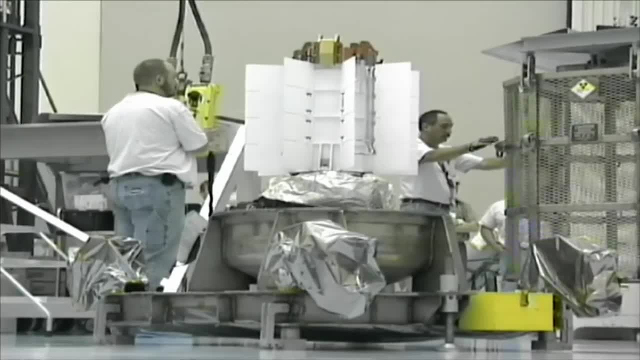 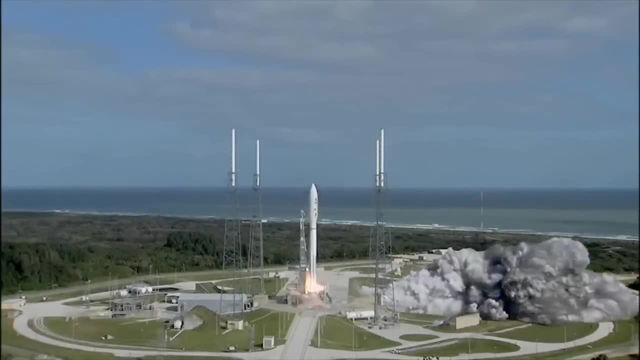 There, an INL team helps NASA personnel unpack the RTG, attach it to the rover and conduct another round of tests before launch And liftoff.